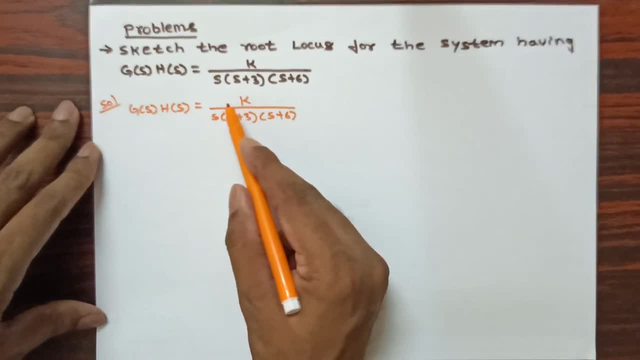 As we know, in open loop transfer function numerator s terms are considered zeros and denominator s terms are considered poles. In this problem, only denominator s terms are given, ie 3 poles are given in this. One pole is s is equal to 0, the another pole is s plus 3 is equal to 0, and the third pole is s plus 6 is equal to 0. 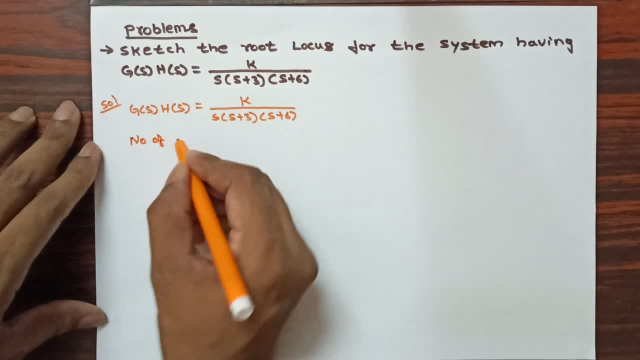 Therefore, number of poles are 3.. That is, s is equal to 0, s plus 3 is equal to 0 and s plus 6 is equal to 0. This can be written as: s is equal to 0, s is equal to minus 3, s is equal to minus. 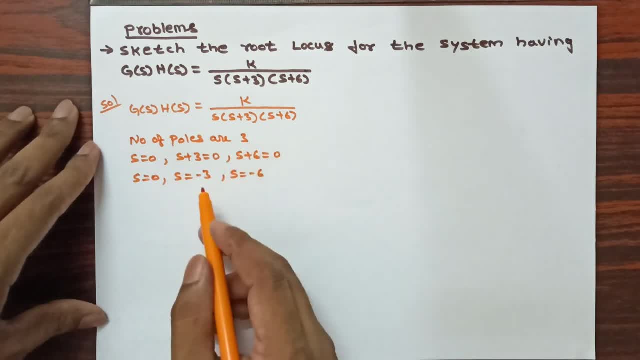 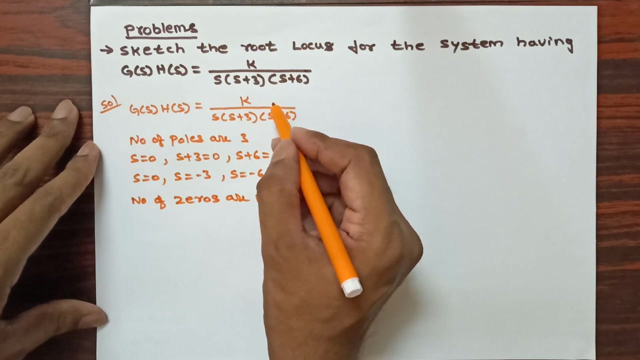 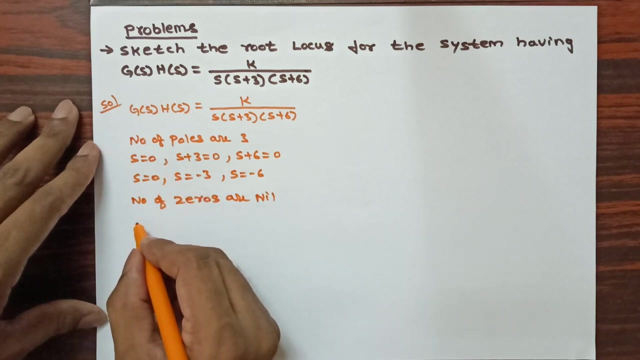 These are the 3 poles given in the problem. Next, number of zeros are nil. In this problem, numerator s terms are not given. That is, 0 is not given in this problem. Therefore, number of zeros are nil. From this we can see number of poles are greater than number of zeros. 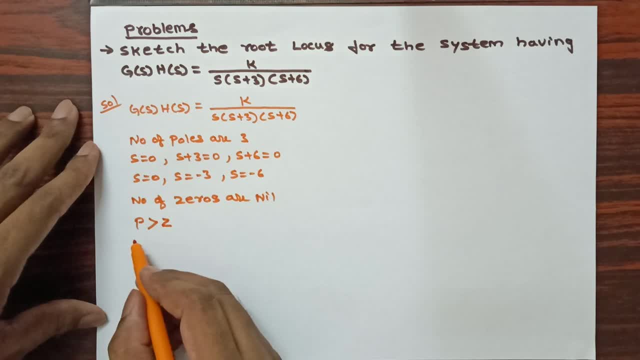 Number of poles are greater than number of zeros. Therefore, we are going to consider number of poles equivalent to number of branches. Number of branches are denoted by capital N. Number of branches, capital N, is equivalent to number of pole, is equivalent to 3.. 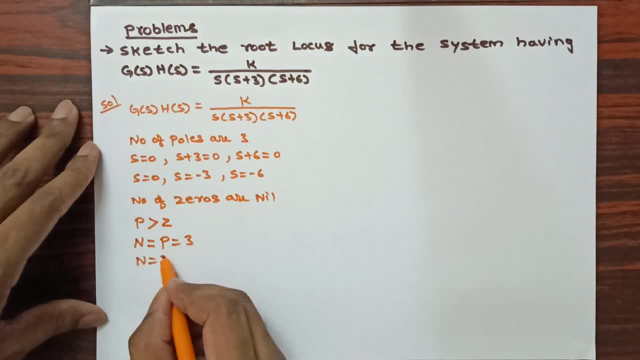 So therefore, we got in this number of branches. N is equal to 3.. Next we are going to plot the number of branches. Next we are going to plot the pole 0 plot- and then we are going to identify the root locus path. 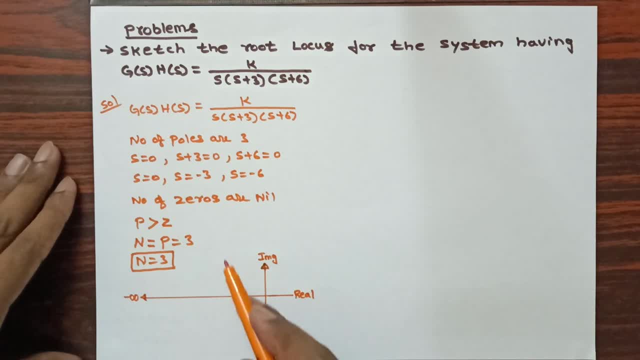 On this real axis. we are going to consider the pole location. You can see here the first pole is: s is equal to 0. That is, at the origin, s is equal to 0. And next pole is s is equal to minus 3.. 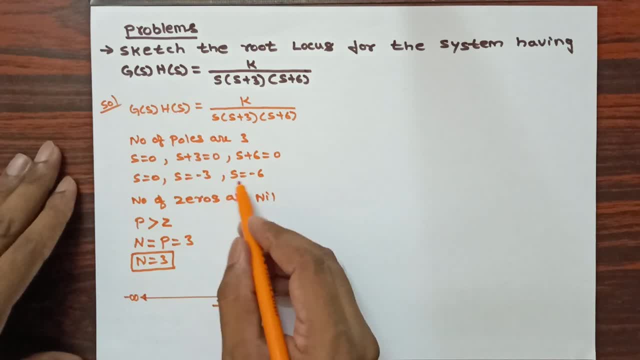 s is equal to minus 3.. And the next pole here, the third pole, is s is equal to minus 3.. And the third pole is s is equal to minus 6.. So now we are going to consider in this root locus path and no root locus path. 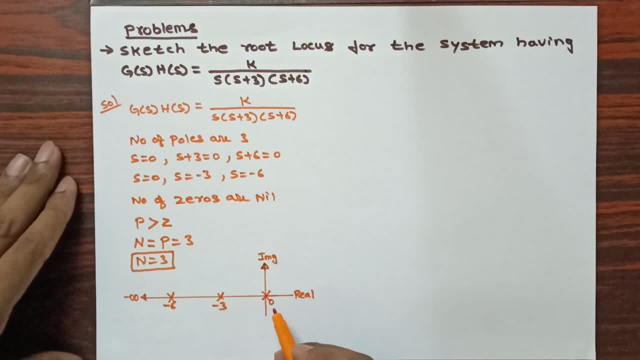 So we know the condition to identify the root locus path is: we are going to consider the root locus path for odd count of poles are zeros And we are going to consider the no root locus path for even count of poles are zeros. In this we can see that from this right hand side, from this point to this point. 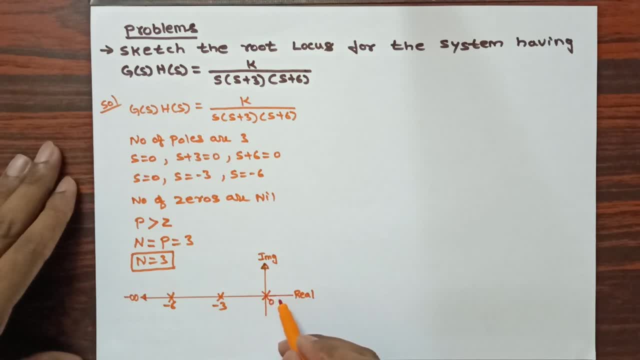 I am not having any possible thing. pole are zero. it is an zero count. zero is an even. therefore, for an even count, i am considering no root locus path. now, at this point we got one pole that is one is an odd. from this pole onwards we 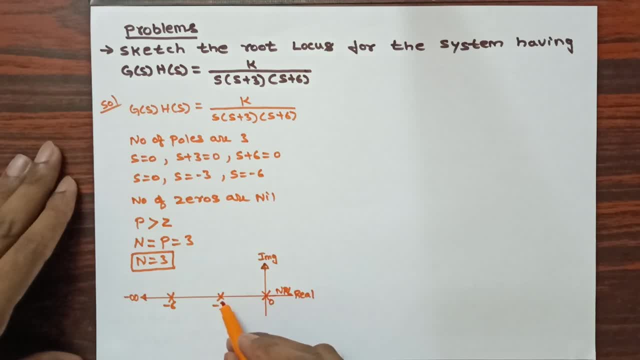 are going to consider the root locus path till next counter. so from this odd count onwards, we are going to consider the root locus path till next counter. so this is an root locus path. and here you can see. now this count becomes two, and two is an even count. next for an even count, we: 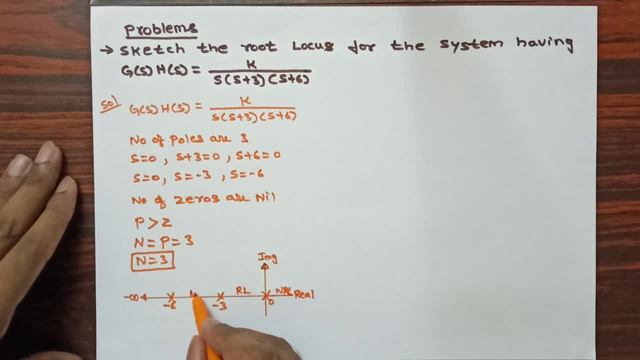 are going to consider the no root locus path till next counter. so here this part is no root locus, till here. now this count becomes three. now three is an odd count and from this odd count onwards we are going to consider the root locus path till next counter. but here we can see that till 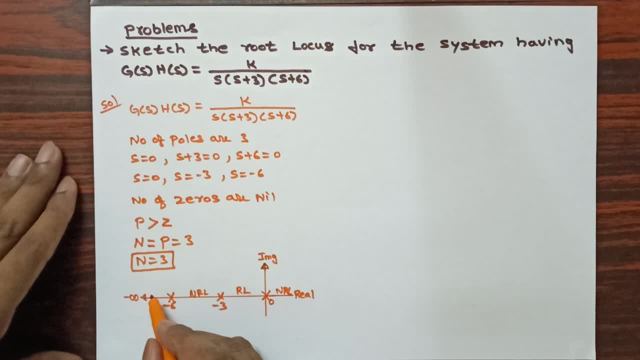 infinity. i am not having any count. therefore, till infinity, it will be considered as root locus path. in this way, we have identified the root locus path now. next we will see the number of branches approaching to infinity. the procedure to identify the number of branches approaching to infinity is: number of poles minus. 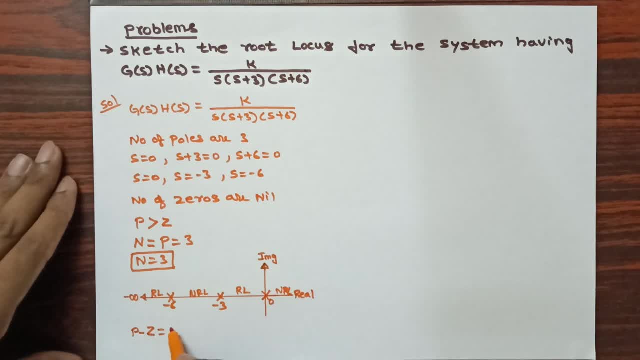 number of zeros is equivalent to number of poles are three in this minus zero, or nil zero. three minus zero. three branches are approaching to infinity, so in this you can see number of poles minus number of zeros. that is equivalent to: in this you can see number of poles minus number of zeros. 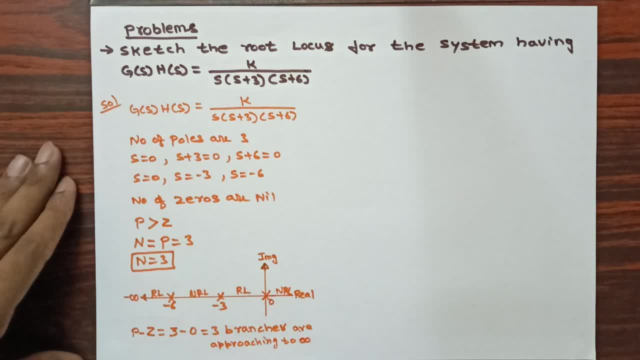 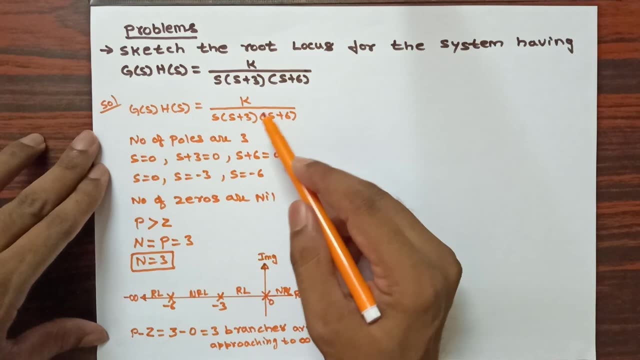 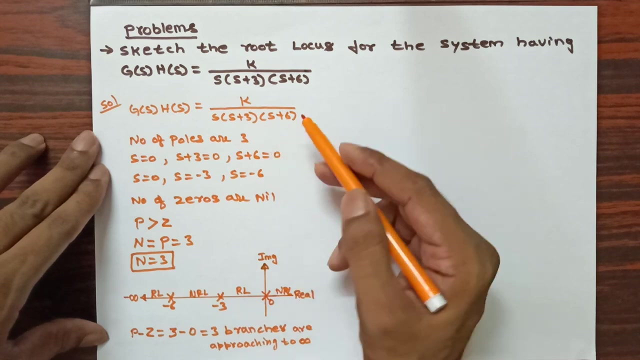 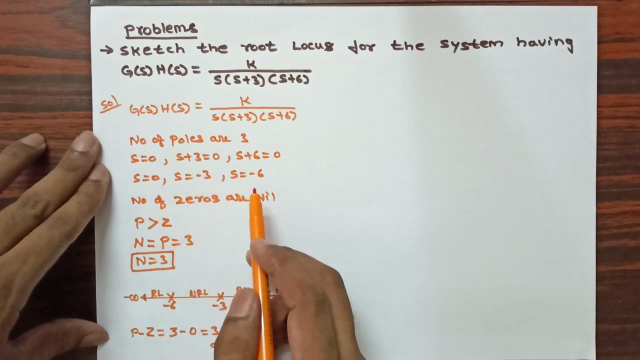 equivalent to three minus zero, that is, three branches are approaching to infinity. in this problem, three poles are given and zeros are not given to end for this poles. therefore, these three poles going to approach to infinity. so in this we know that the starting points are zero minus three and minus six and for this starting points, the ending points are infinity. 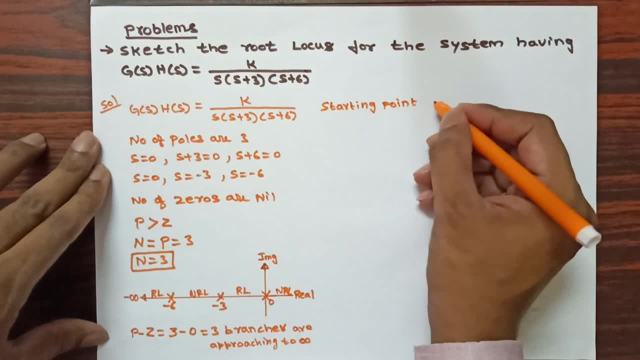 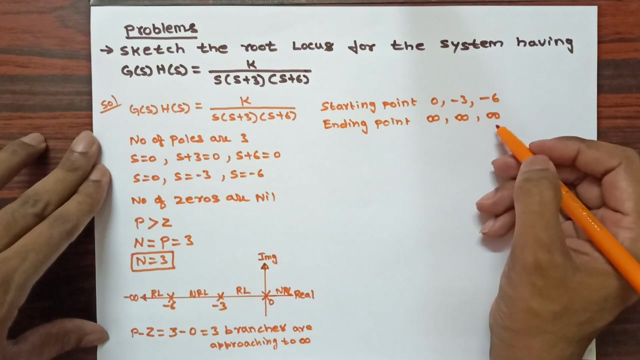 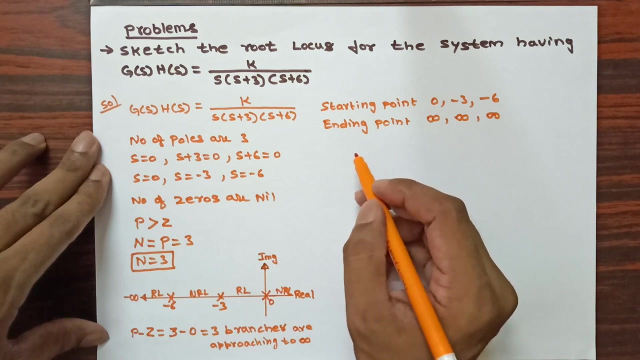 starting point: zero minus three, minus six. ending point: infinity, infinity, infinity. for this start pole, the end is infinity. and in this, for start pole, end point is infinity, and for this start pole also, the end point is infinity. when these three branches are approaching to infinity, we need to provide an angle for these three branches, and such angle we call angle of asymptotes. next we 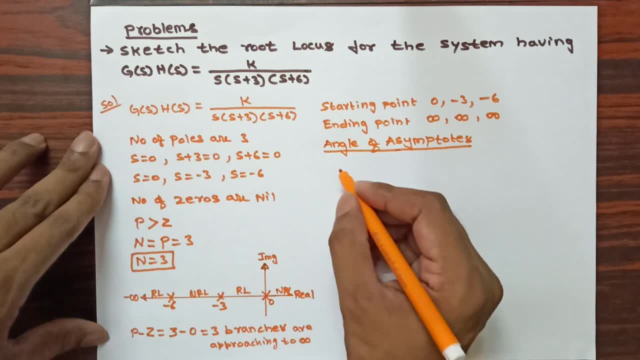 are going to calculate angle of asymptotes, and the formula to calculate angle of asymptotes is: theta is equivalent to 2 q plus 1 into 180 degree divided by number of poles minus number of zeros, and here this q value changes depending upon the number of poles. in this we need to find three angles. three angle: 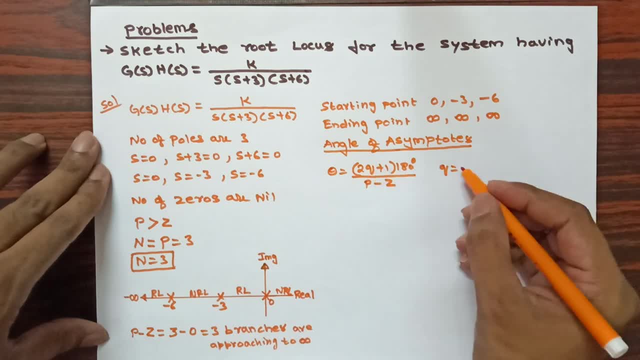 of asymptotes, therefore the q value. initially we are going to consider 0 for first angle. then i am going to substitute q is equal to 1 to get the second angle, and next i am going to substitute q is equal to 2 to get the third angle. in this formula now we will: 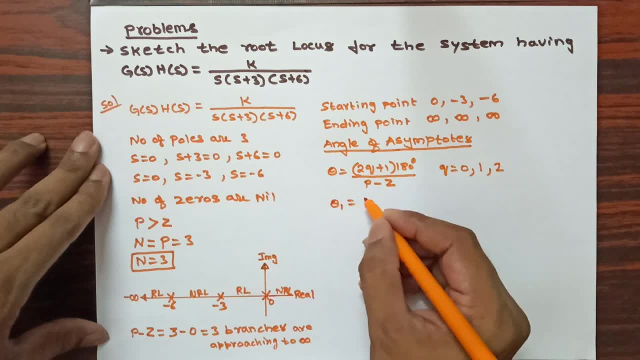 consider first: q is equal to 0, theta 1 is equivalent to 2 into q is equal to 0 plus 1 into 180 degree. divided by number of poles are in this case 3, 3 minus number of zeros are nil zero. now here: 2 into 0, 0, 0 plus 1, 1, 1 into 180. 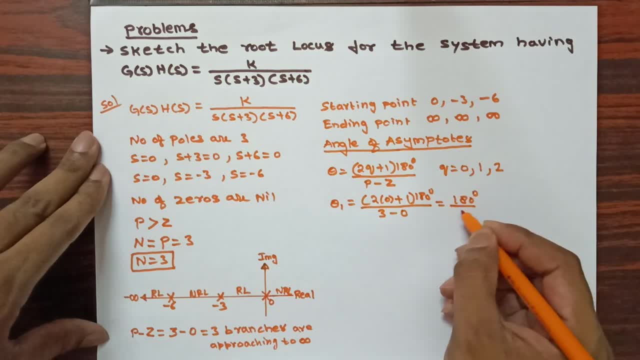 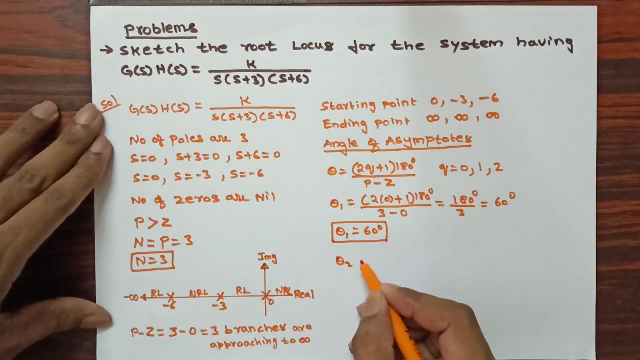 degree divided by 3. 180 degree divided by 3 is equal to: here we are getting 60 degree. so therefore we got the first angle. theta 1 is equal to 60. next, to calculate the second angle, theta 2 is equal to 2 into q. this time I am going to substitute now 1 plus 1 into 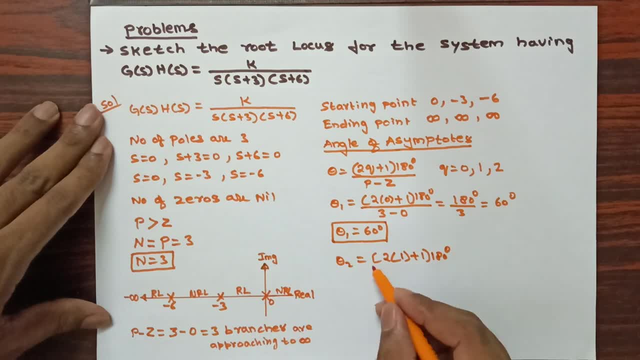 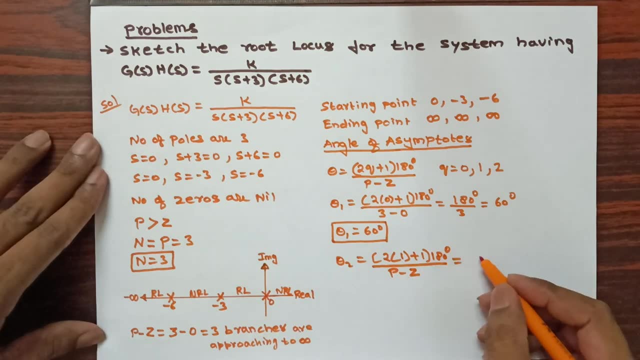 180 degree. divided by number of poles minus number of zeros, this will be equivalent to 1, 2, 2 plus 1, 3. 3 into 180 degree. 540 degree divided by number of poles are 3, 3 minus number of zeros, 0. here we are getting: 3 is equivalent to 540 degree. divided by 3 is 180 degree. in this way, 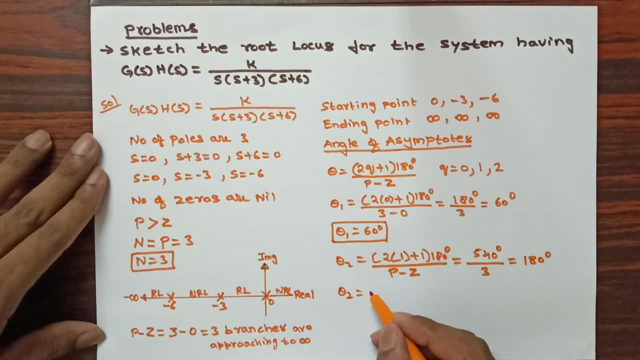 we got the second angle- theta 1 is equal to 3- into q- this time I am going to substitute into 0, zero, and now we have completed 2, so we have 2 square and these two are equal to 0. that is 2 by 4, where. 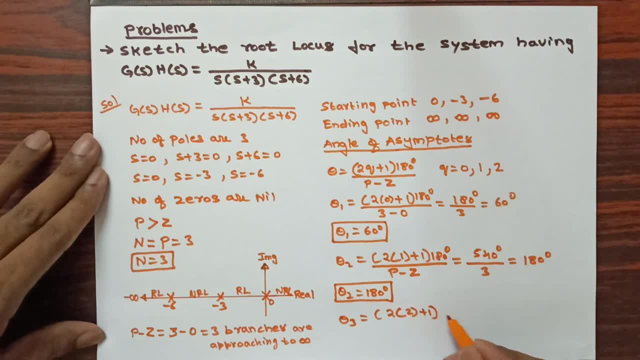 now the first angle: theta 1 is equal to 2 into 180 admitted angle, and the last angle we are getting 534 degree. theta 2 is equal to 6, party care 0. this will be equivalent to 2 into 2, 4, 4 plus 1, 5, 5 into 180 degree, 900 divided by 3 minus 0, 3. 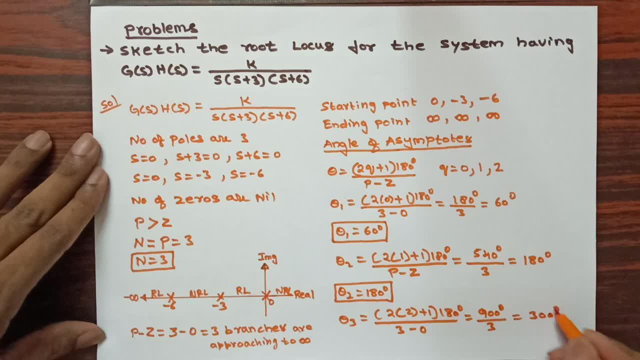 this will be equivalent to 300 degree. we got the third angle. theta 3 is equivalent to 300 degree. now, these three angles we are going to draw on the real axis of the s plane. to draw these three angles on the real axis, i need a point which we called centroid. next we will calculate the 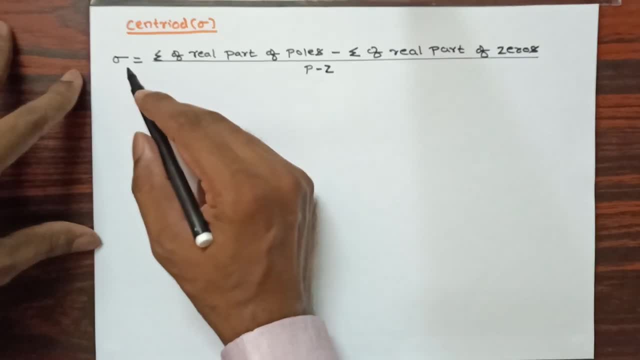 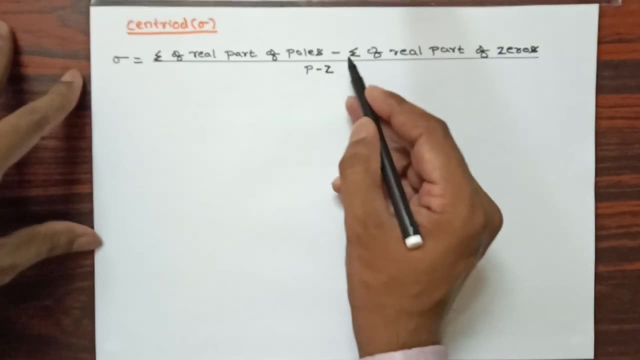 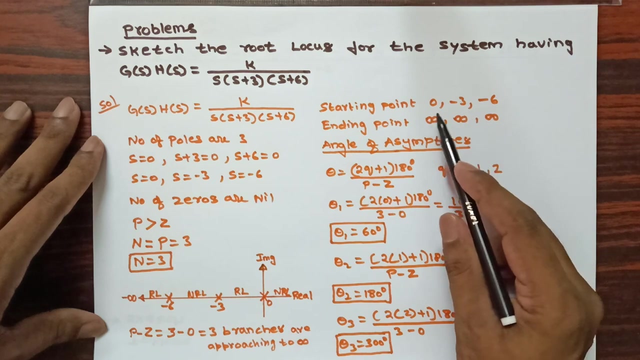 centroid, centroid denoted by sigma. we know the formula for a centroid sigma is equivalent to summation of real part of poles minus summation of real part of poles, real part of zeros divided by number of poles minus number of zeros. in the problem, the pole values are 0 minus 3 minus 6. summation of this real part of pole- 0 minus 3 and minus 6, is going: 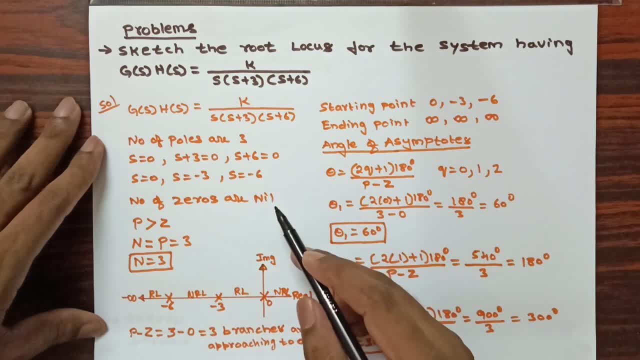 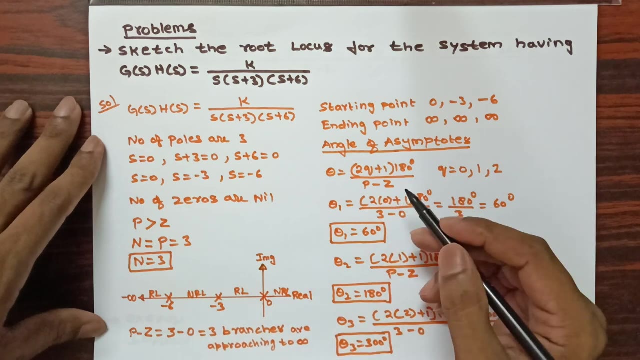 to be substituted in the formula to calculate centroid. and the second part, summation of real part of zeros. in this problem zeros are nil and in the denominator number of poles are 3 minus number of zeros are nil. so by substituting these values we are going to calculate the centroid. 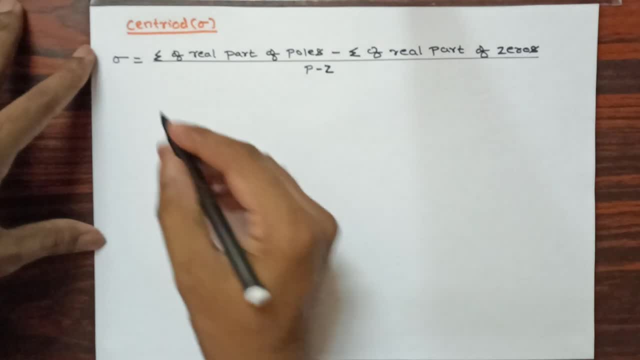 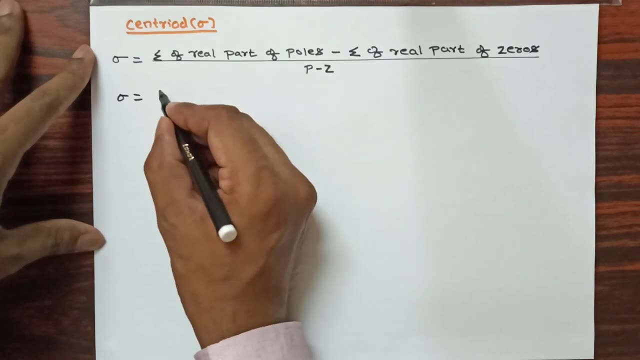 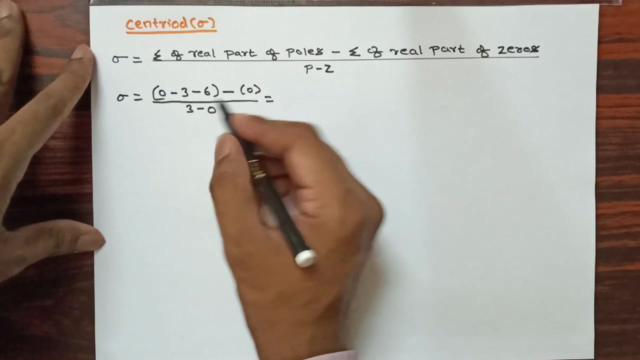 sigma is equal to summation of real part of poles, that is, 0 minus 3 minus 6. these are the real part of poles minus real part of 0 in this problem is 0. this, divided by number of poles, are 3 minus number of zeros are 0. therefore, I'm getting here minus 3. 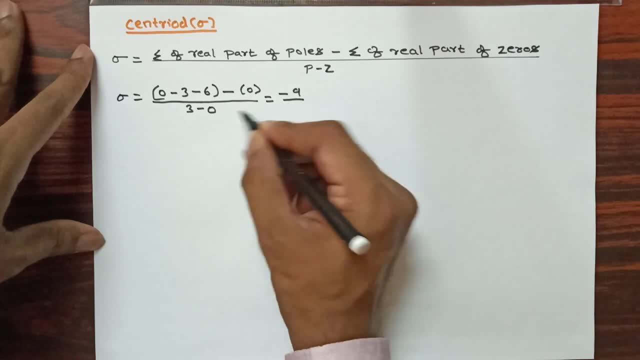 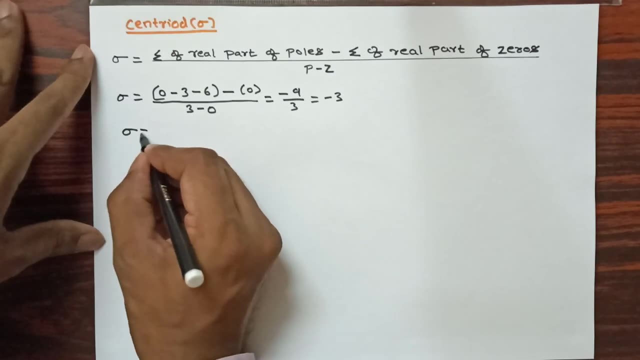 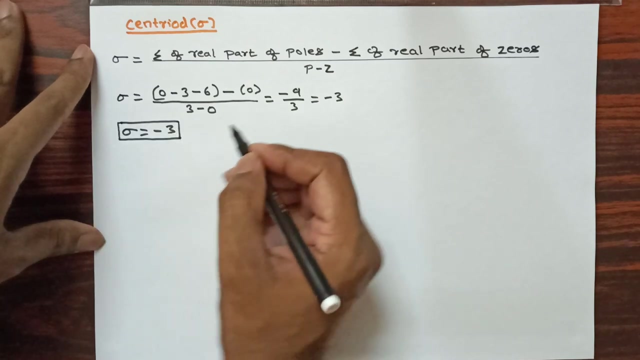 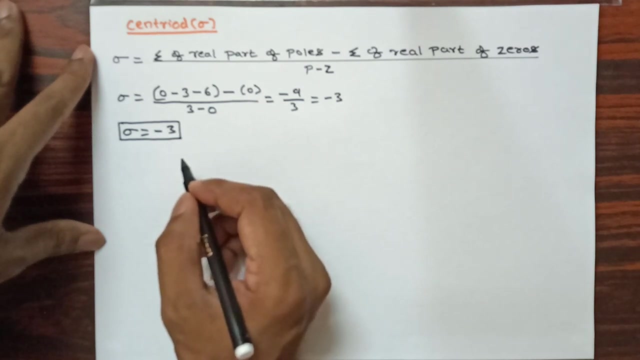 minus 6 minus 9. divided by 3 minus 0, 3, this will be equivalent to minus 3. so here we. I got the centroid value minus 3. next we are going to calculate the breakaway point in this problem. we are having more than one branch, therefore we may get a breakaway point, so we are going to 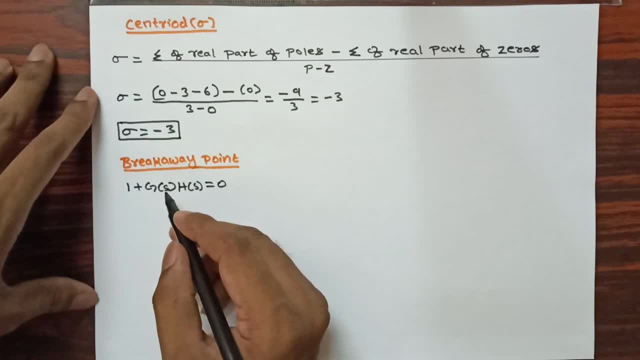 calculate the next breakaway point. so to calculate a breakaway point, we are going to consider first characteristic equation that is 1 plus g of s into h of s is equal to 0. we know, g of s into h of s, that is k divided by s into s plus 3, into s plus 6, by substituting: 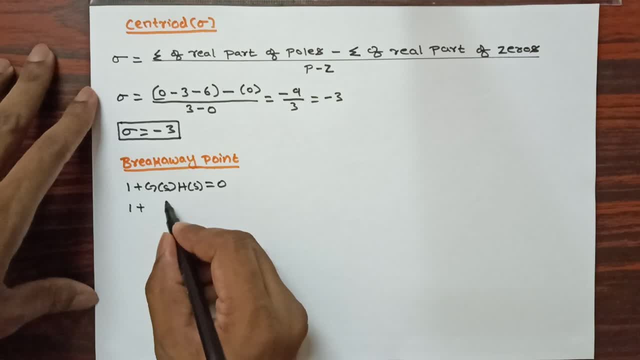 that value in this 1 plus k, divided by s into s plus 3, into s plus 6, is equal to 0. by taking the LCM we are going to get s into s plus 3, into s plus 6 plus k. whole, divided by s into s plus 3, into s plus 6, is equal to 0. this denominator 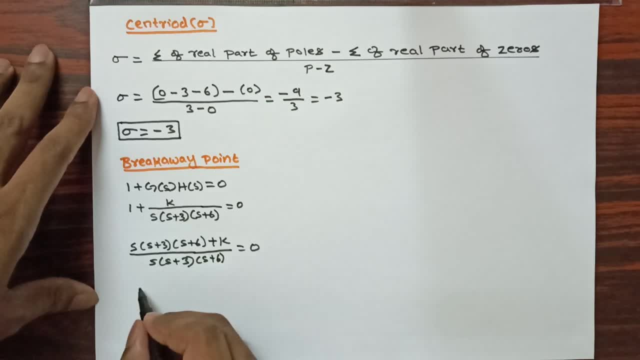 term goes to the right hand side becomes 0, then I will get s into s plus 3 into s plus 6 plus k is equal to 0. by multiplying this value I will get s to the power 3 plus 9 s square plus. 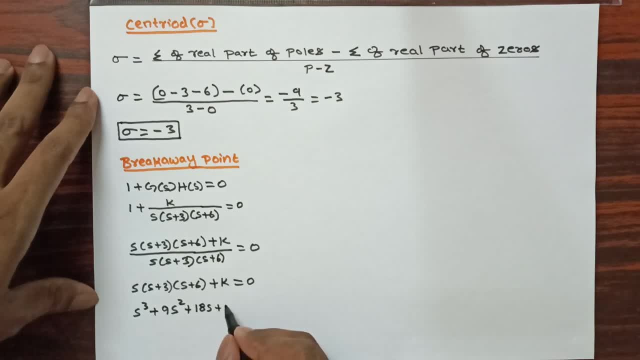 18 s plus k is equal to 0. now, once I get the characteristic equation, the next step to find the breakaway point is: I am going to find the k equation. I am retaining k in the left hand side and I will take all s terms to the right hand side. k is equivalent to: 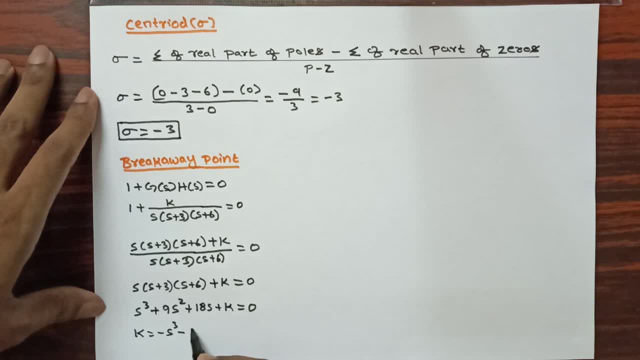 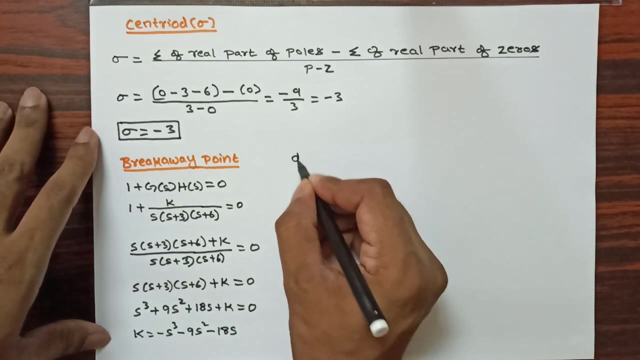 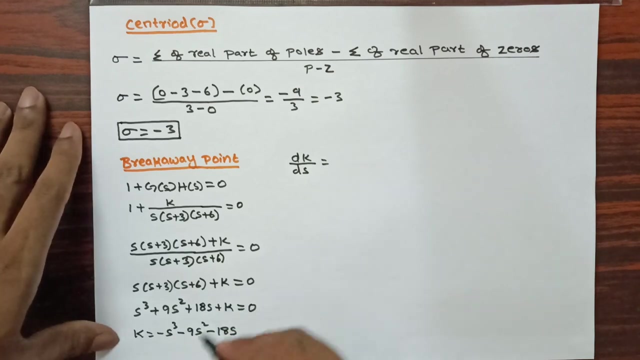 minus s to the power 3 minus 9 s, square minus 18 s. so now for this k equation. we are going to differentiate with respect to s dk by: ds is equal to. we are going to take equal to. I s equal to less than or equal to 0. so this period it. 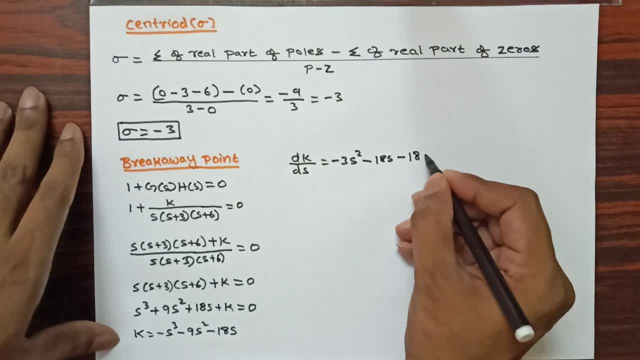 is going to be byalon root. so our differential equation is negative. K root x squared, This food, denoted by 2s, measured, which is equal to minus 3sア, square minus. different situation of 9: square is 18? yes, minus if differentiation of 18 s equals 0. here I got the differentiated equation-3要 żeby0-3. 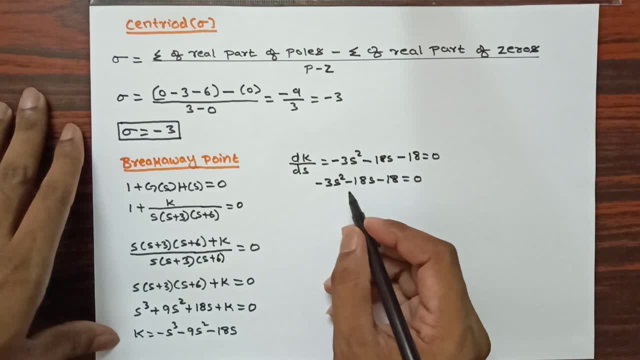 is equal to 0.. we'll find the root values of this equation here. the power is 2, then i'm going to get two root values in this i'm getting. s is equal to minus 1.26 and the second root value i'm getting. 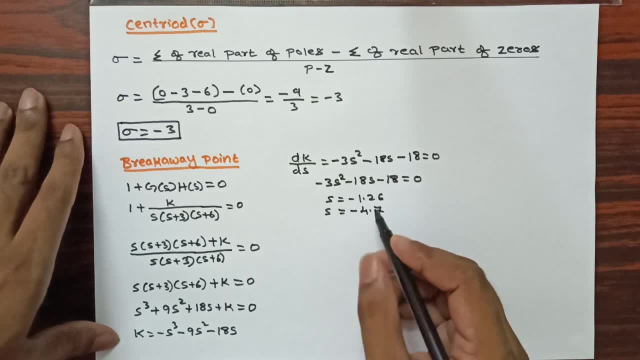 s is equal to minus 4.7. these are the two values i got. these are the breakaway points. now i need to check whether these two breakaway points are valid. breakaway points are invalid breakaway points. to check the validity of the breakaway point, i need to substitute this s value in this. 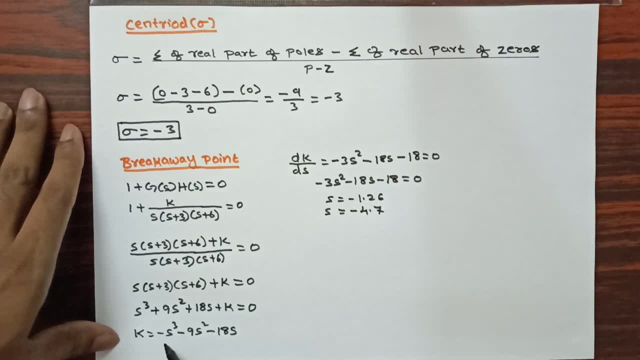 k equation. now, after substituting: if i get the k value positive, then that s value is a valid breakaway point. if i'm getting negative k value, then that s value is invalid breakaway point. so first we are going to substitute: s is equal to minus 1.26, and then s is equal to minus 1.26. 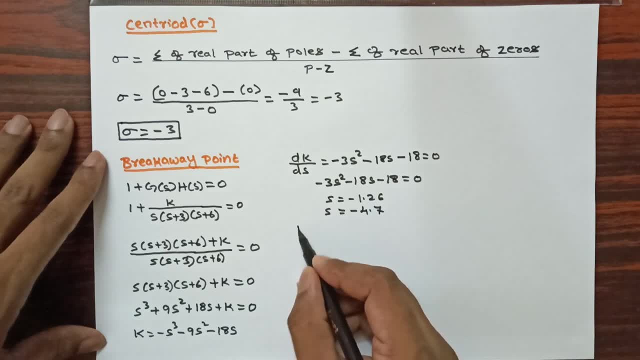 1.26 and we'll see what k value we are going to get. k is equivalent to minus s, to the power 3 minus 9 s, square minus 18 s. for this i'm going to consider first. s is equivalent to minus 1.26. 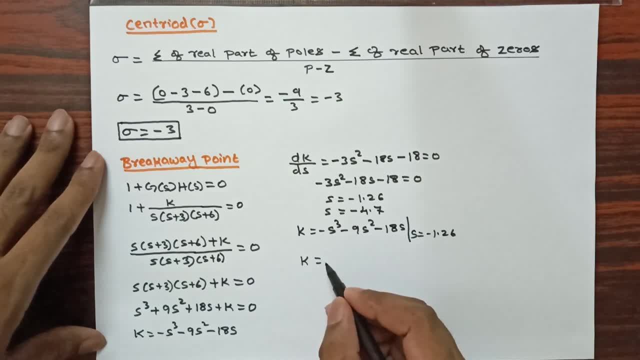 for this. i am getting here k value 10.39. you can see here i'm getting a positive value. therefore, the s value is: therefore: s is equal to minus 1.26 is valid. breakaway pointer: minus s is equal to minus 1.26 is valid. 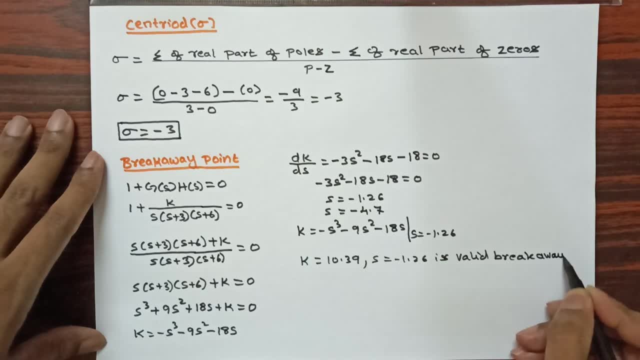 breakaway pointer next we are going to check for: s is equal to minus 4.7, k is equivalent to minus. s is equal to minus 1.26, k is equivalent to minus s to the power 3 minus 9 s. square minus 18 s. 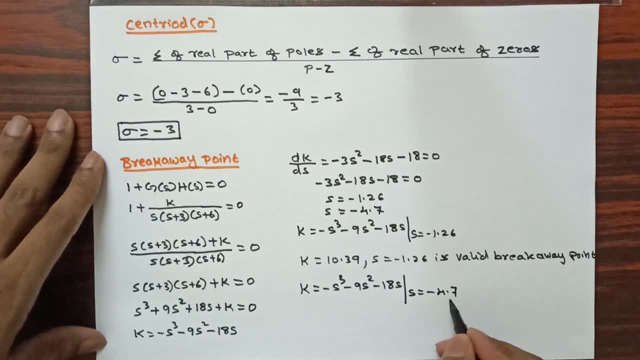 s is equal to minus 4.7. by substituting minus 4.7 in this s, by substituting this s value minus 4.7 in this equation i am getting: k is equivalent to minus 10.39. so in this you can see. 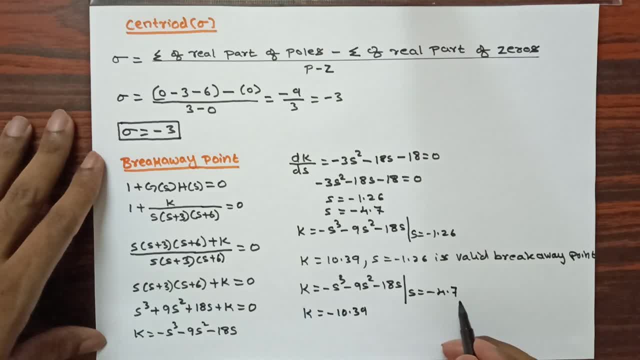 i am getting negative k value. therefore, s is equal to minus 4.7 is invalid breakaway pointer. s is equal to minus 4.7 is invalid breakaway point. in this way, we are going to check whether the breakaway points are valid or invalid. remember if 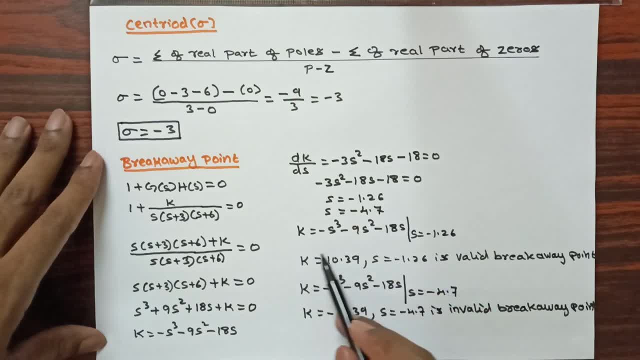 breakaway points are real, then we are going to check by this method, by considering the k equation. if breakaway points are complex, then we are not going to check by this k equation. we are going to use angle condition and magnitude, condition that i will discuss in. 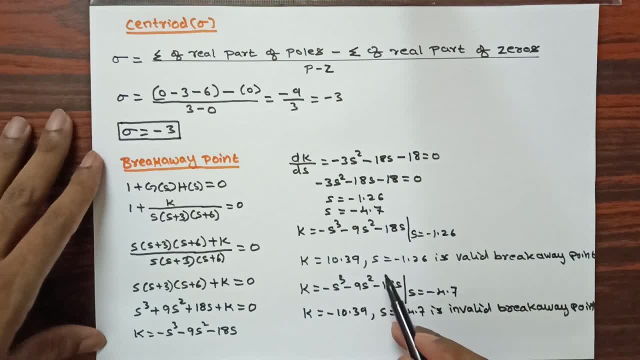 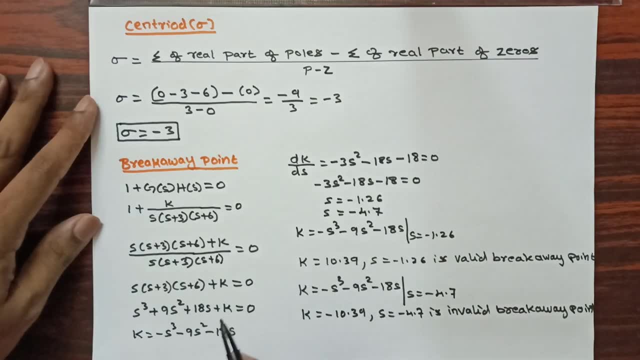 the other problems in this. i got one valid breakaway point that is: s is equal to minus 1.26. from this we have understood that to find the breakaway point first we need to find the characteristic equation. from this characteristic equation we are going to form the k equation and 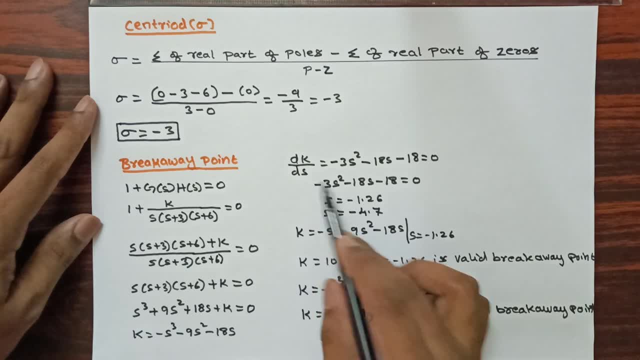 for this k equation, we are going to differentiate with respect to s, then we are going to get the differentiated equation. from that we are going to calculate the root values, that is, the breakaway point values, and then we will check the validity of this breakaway points by substituting in k. 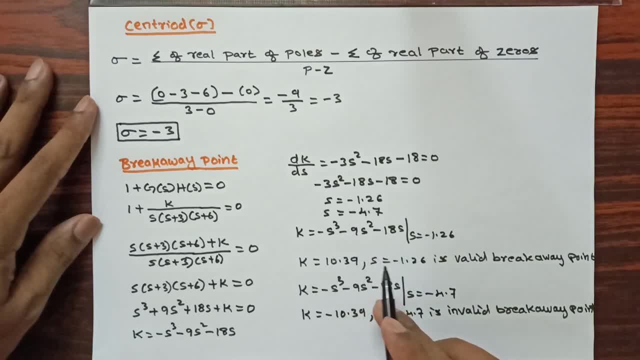 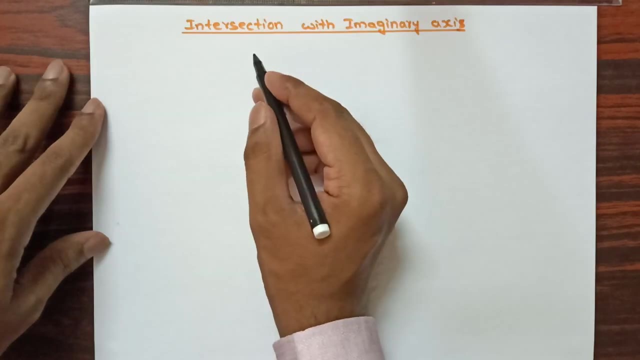 equation: if k is positive, then it is, then it will be a valid breakaway point. if k value is negative, then it will be a invalid breakaway pointer. next, we are going to calculate the intersection with imaginary axis. to calculate intersection with imaginary axis i need to consider here roots array. 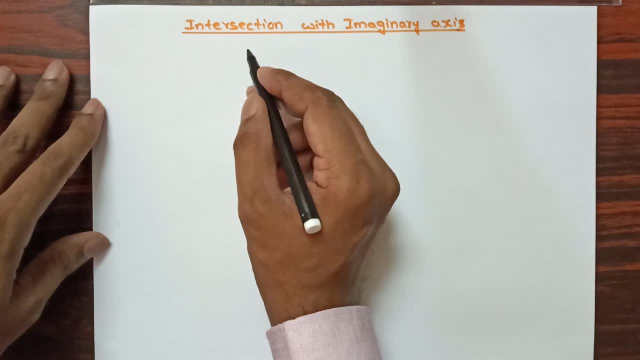 method, that is, i need to get the characteristic equation. from that characteristic equation i am going to form the route array and then from that we are going to calculate k margin and frequency of sustained oscillation. that is a intersection with imaginary axis. First I need to consider in this intersection with imaginary axis, 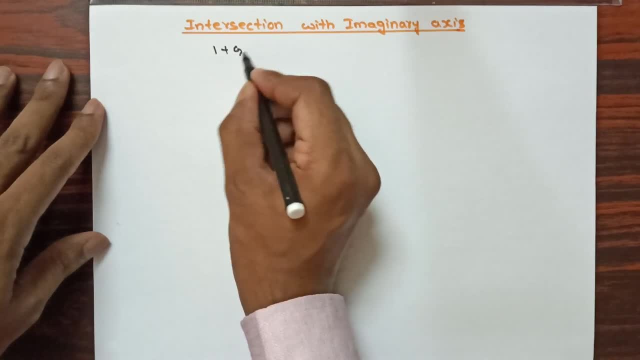 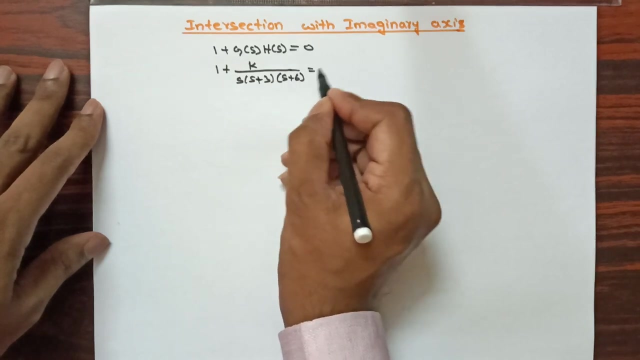 is characteristic equation that is, 1 plus g of s into h of s is equal to 0.. As we know, the characteristic equation, as we know, g of s into h of s value, 1 plus k, divided by s into s plus 3 into s plus 6, is equivalent to 0.. By taking this LCM and by substituting, we get the characteristic. 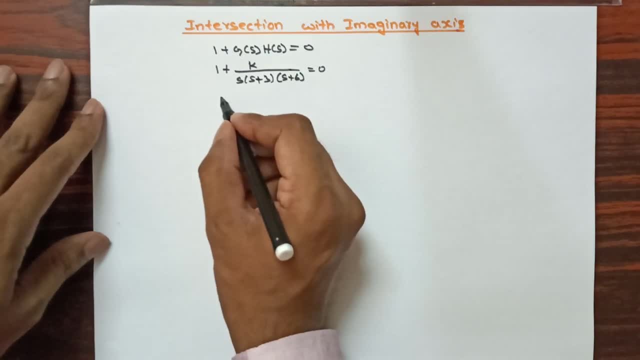 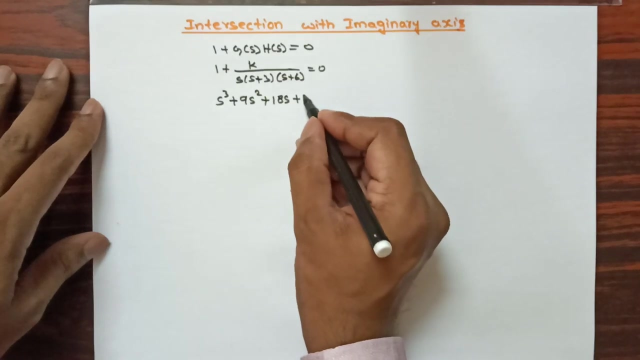 equation Just now. we have calculated in the breakaway point the characteristic equation I will get by simplifying this is: s to the power 3 plus s to the power 3 plus 9, s to the power 2 plus 18, s plus k is equal to: 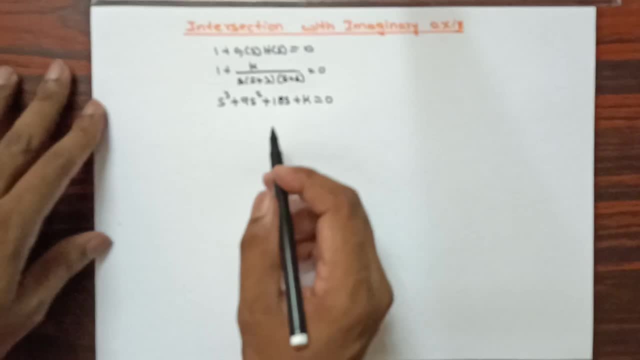 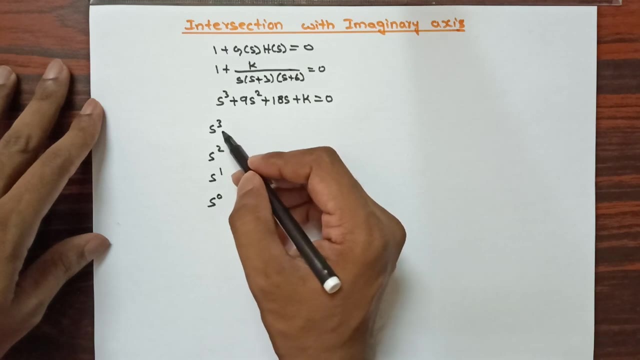 0.. This is the characteristic equation I got For this. we are going to form the array. The highest power is s to the power 3.. I have considered that first, s to the power 3 and next I have considered the s power in decrementing order, that is, s to the power 2, s to the power 1, s to the power 0.. 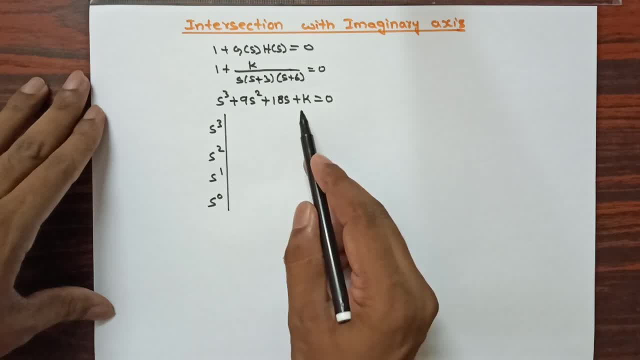 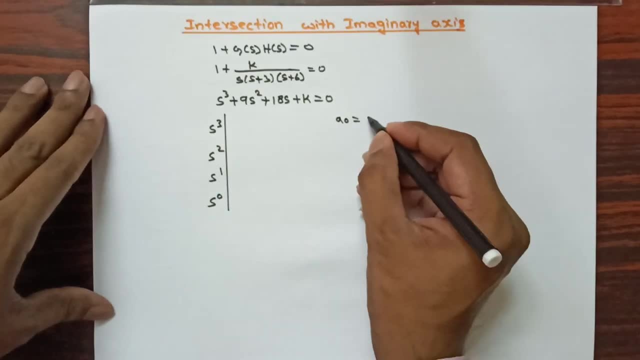 Next we are going to form the two rows from this characteristic equation. For that we know that first coefficient, a naught is a naught is equivalent to 1 and 8, 1.. A1 is equivalent to 9 and then a2 is equivalent to 18.. A3 is equivalent to k. These are the 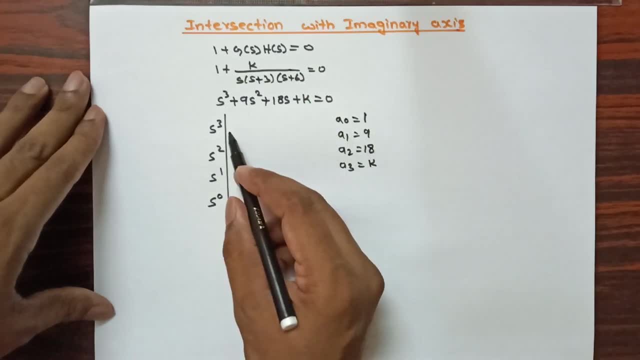 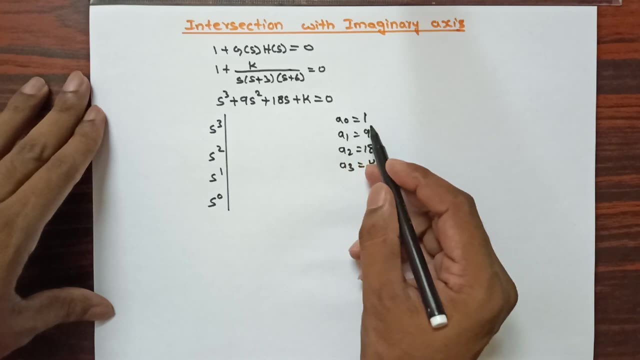 coefficients in the characteristic equation, For in the first row I am going to consider the even coefficient, that is, a naught and a2, and this coefficients values are 1 and 18.. So in the first row I am going to write 1 and 18 and 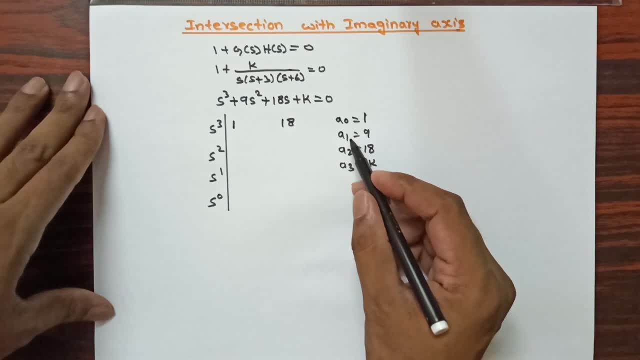 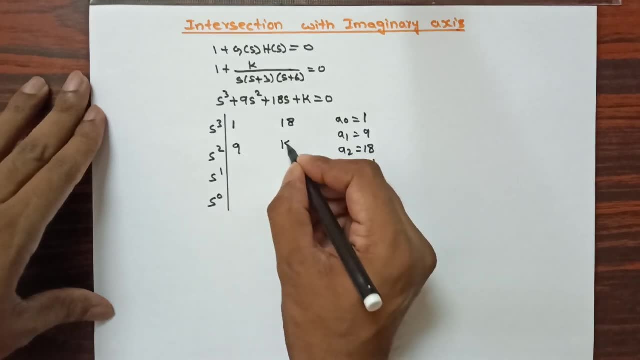 to form the second row, I am going to consider the odd coefficients, that is, a1 and a3, and a1 value is 9 and a3 value is k, 9 and k. and the third row we are going to form by multiplying 9 into 18.. We are 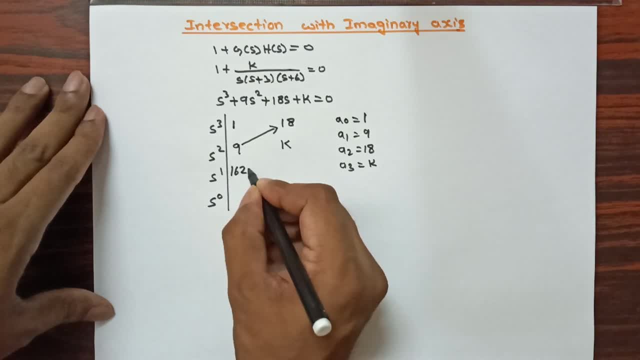 getting here: 9 into 18 is 162 minus 1 into k, 1 into k divided by 9. and next I am not having any coefficient, Therefore here I will get 0.. So to get the fourth row, I am going to multiply this term with k minus 9 into 0.. 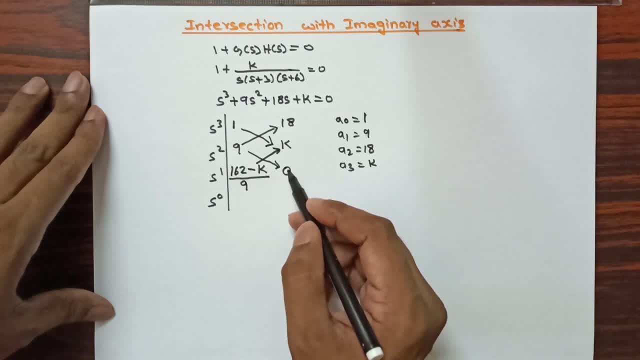 As we know, if we have in the diagonal 0, then the resultant value is above value, that is k. That directly I can write here in the fourth row: k. Now from this we are going to find the k margin value For that. we know that first we are going to consider s to the power 0 row, from s to the power 1.. 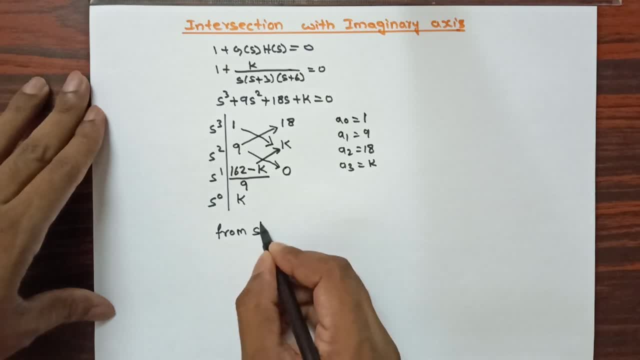 So we are going to write from s to the power 0 row, from s to the power 0, that is, from s to the power 0. k is greater than 0.. Next, from s to the power 1, this equation, 162 minus k divided by 9, equal to 0.. Now, 162 minus k divided by 9 is equal to 0.. 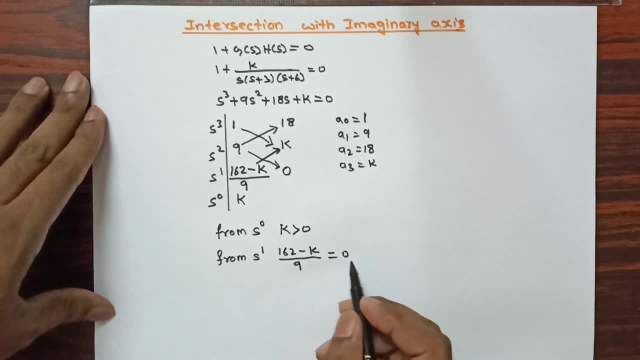 This 9 goes to right and side becomes 0.. 162 minus k is equal to 0. Here, therefore, k, we are getting 162, which is nothing but k marginal value. Here we got the k marginal value 162.. Now we are going to consider the auxiliary equation. 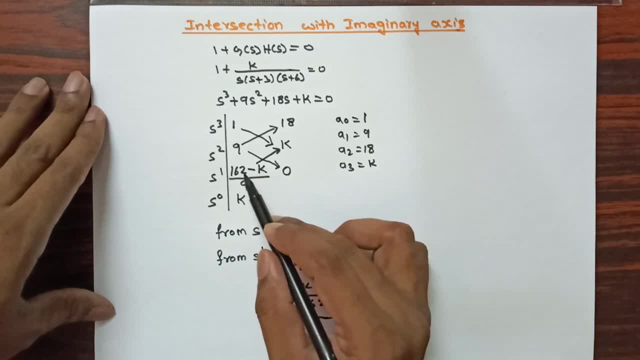 If I substitute this k value in this, This whole row becomes 0.. The zeroth drvor much another value will be 0 to the power minus 1.. 이스 zero. zero above rho is an axillary equation. by considering an axillary equation, a of s is: 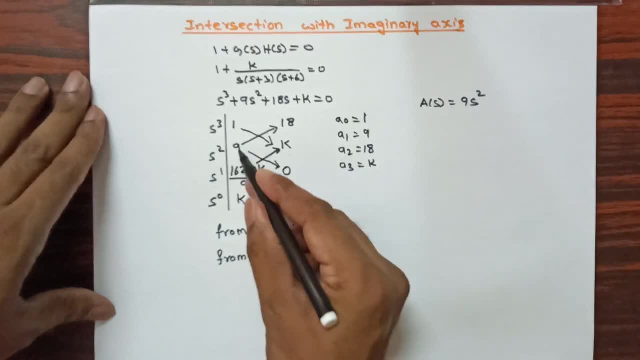 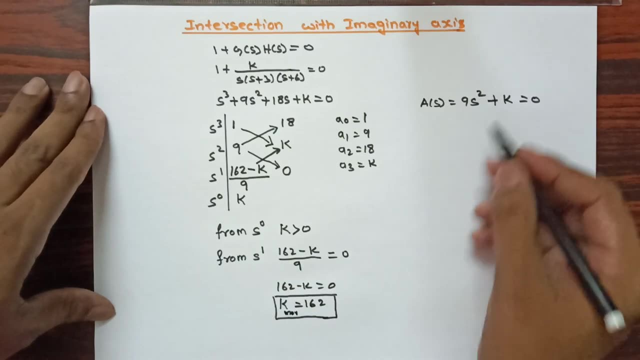 equivalent to 9 s square. 9 s square plus k equal to zero. now we know the k value. k value is 162. we are going to substitute this k value in this axillary equation: 9 s square plus 162 is equal to zero. next, by simplifying this, i'm going to get: 9 s square is equivalent to minus 162. 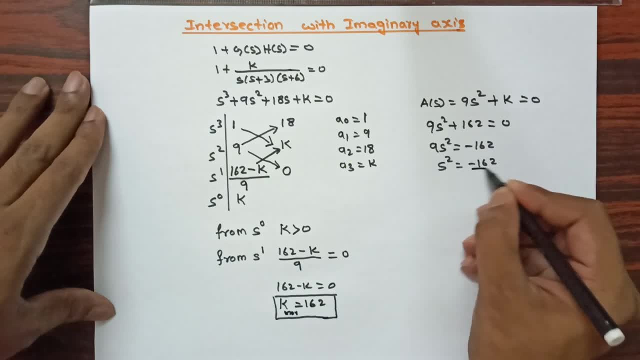 s square is equivalent to minus 162 by 9. s square is equivalent to minus 60, 162 by 9 minus 18, and s is equivalent to square of minus is plus or minus j root of 18, and this will be equivalent to s plus or minus j. 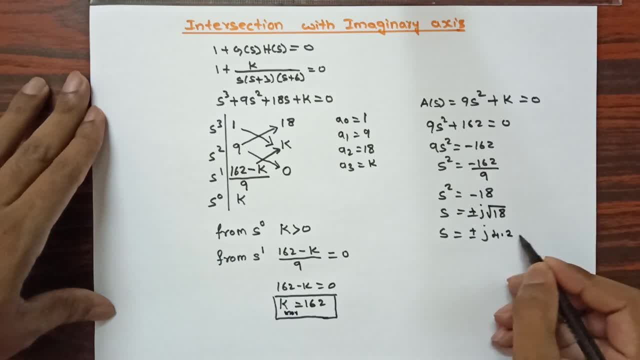 root of 18 is 4.24. this value is the intersection with imaginary axis. that is, we got one s is equal to plus j 4.24, and the below value i got, s, is equal to minus j 4.24. now, by considering: 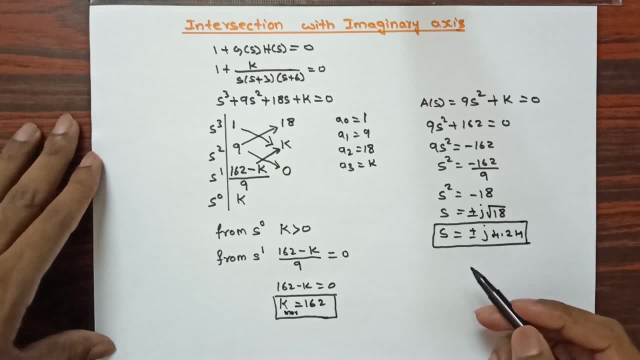 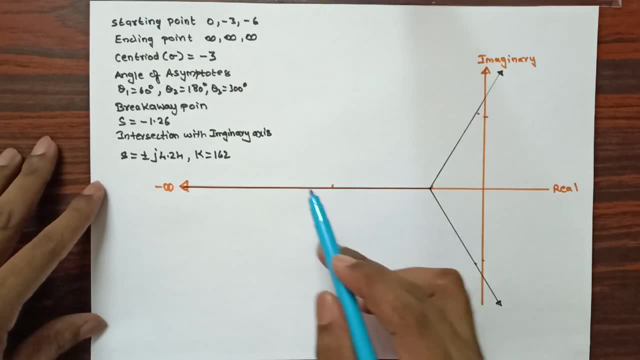 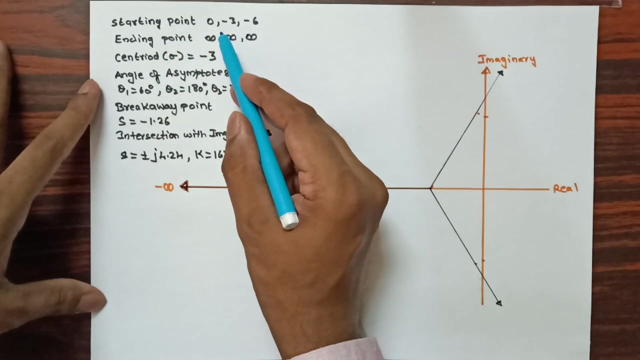 these values, we are going to sketch the root locus. now, to sketch the root locus, we have to consider the graph sheet. for an explanation purpose, i have considered a normal sheet here. you have to draw on the graph sheet. by considering all this calculation, what we have done, that is starting point 0 minus 3 minus 6, ending point. 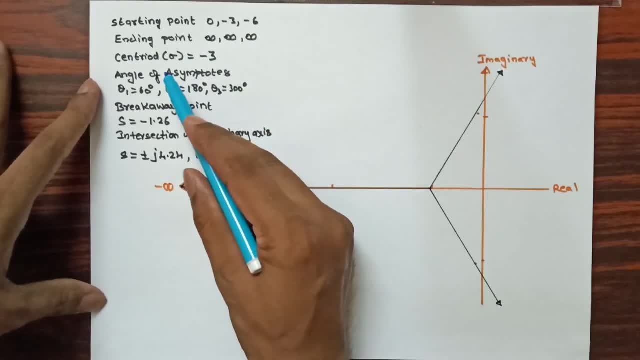 infinity, infinity, infinity. then centroid: we got minus 3 si. then centroid, we got minus 2 locus. so i have to write the locus as e to the square and i have to and angle of asymptotes we got: theta1 is equal to 60 degree. theta2 is equal to 180 degree. theta3. 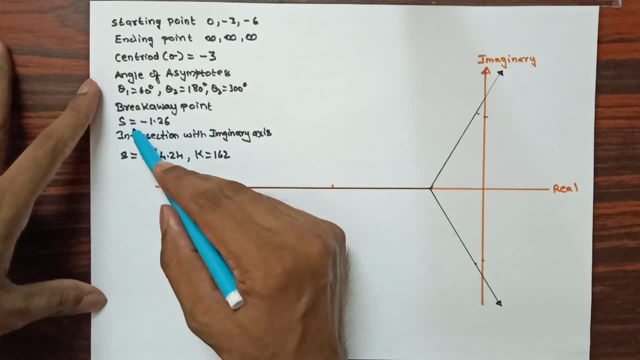 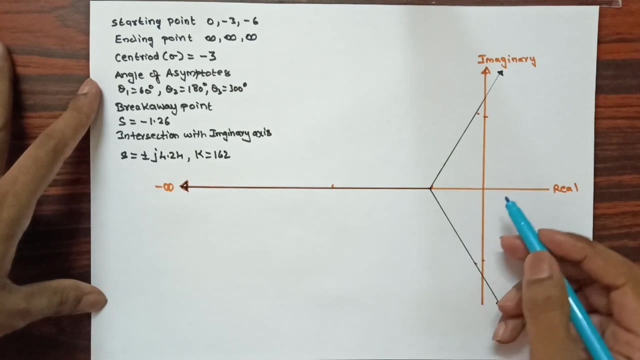 is equal to 300 degree. then breakaway point: we got a valid breakaway point. s is equal to minus 1.26. and then intersection with imaginary axis: we got s is equal to plus or minus j 4.24. for k margin is equivalent to 162. to sketch the root locus, the first step we need to locate the pole. 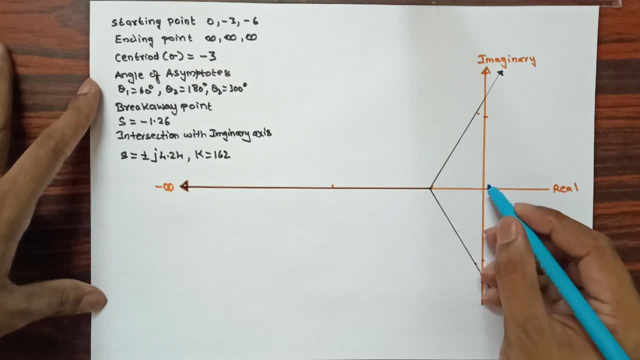 location on this real axis. we know that the first pole is at origin, that is 0, s is equal to 0. and then second pole is at minus 3 and third pole is at minus 6. these are the pole locations. next we are going to identify the root locus path. for that we know the procedure for an odd count. we are going 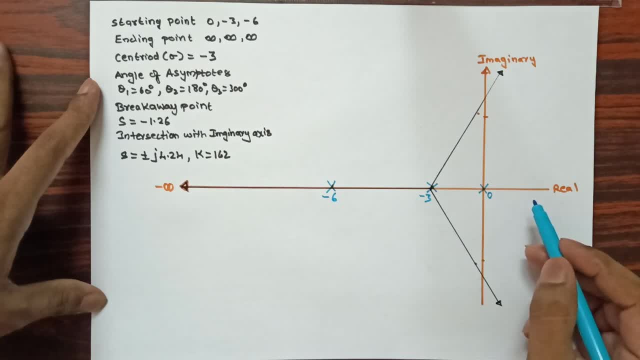 to consider the root locus path and for an even count, we are going to consider the no root locus path. from this point to this point, even count, that is zero count. therefore, we are going to consider no root locus path. at this point the count becomes one. it is an odd count. from this point to next count, we 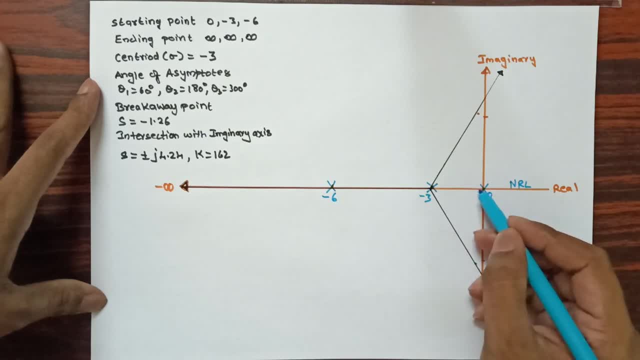 are going to consider the root locus path. so from here to till here, this part is root locus and now, at this point, the count becomes two. from this even count to next count, we are going to consider no root locus path and at this point the count becomes three. now, three is an odd from this. 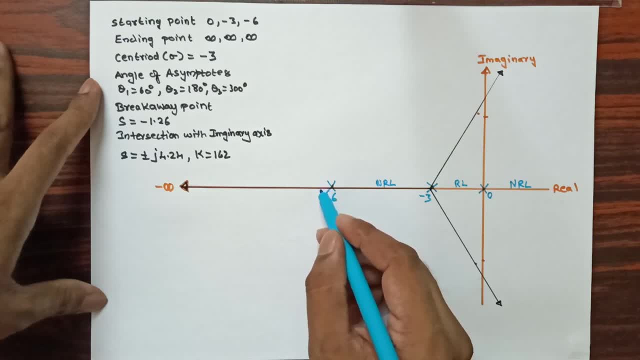 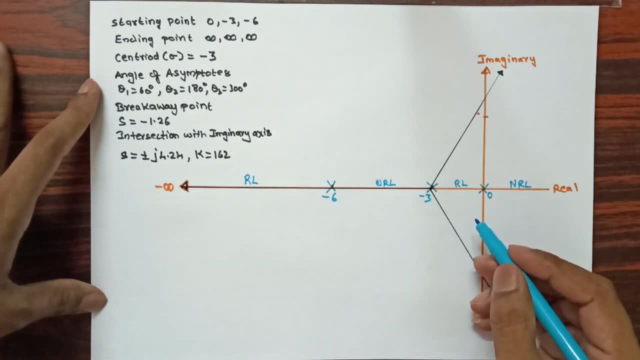 odd count onwards. we are going to consider the root locus path till next count, but here i am not having any count. therefore, till infinity it is root locus path. now, after this, we are going to consider the centroid point, and here we got a centroid point minus three here in this. this is the centroid. 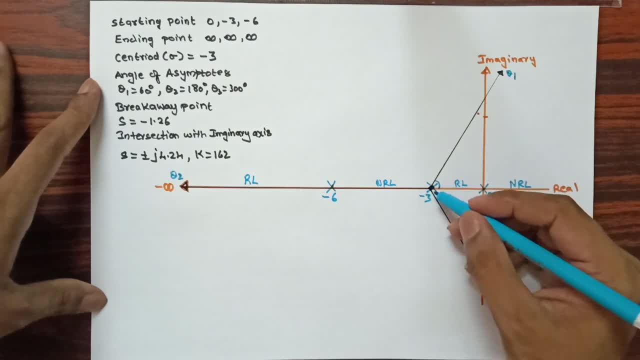 point, that is minus three. i have taken from this point, i have drawn a centroid point, and i have drawn first angle, theta 1, 60 degree, and then second angle, i have considered 180 degree, that is, theta 2. and third angle, i have considered 300 degree, theta 3. in this way we have shown the angle of 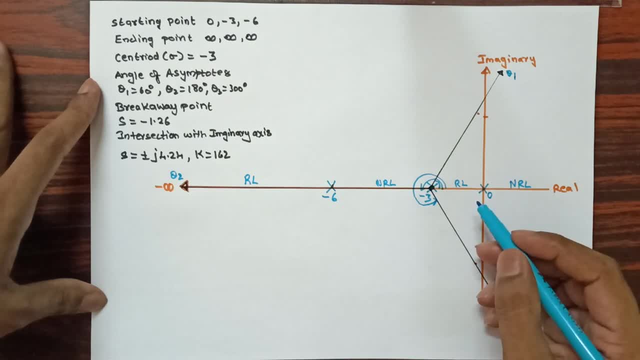 asymptotes. now we know that when i apply the input k is equal to 0 to infinity. this pole will move in root locus path. so this pole will start to move in this direction. and this pole will start to move in this direction. then we can see here this: both the poles, they are going to meet at one point, that we know that a. 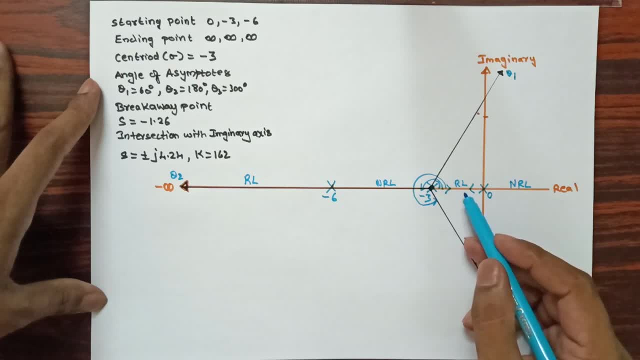 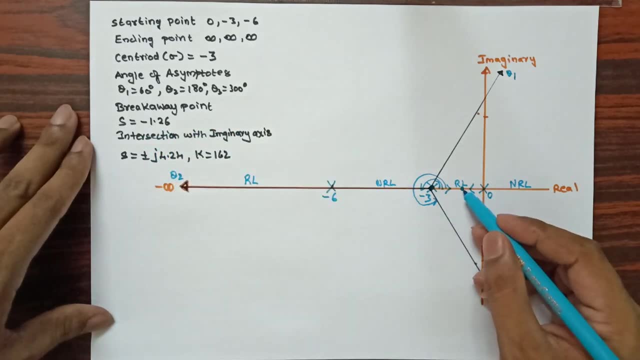 point where more than one branch meets. we called breakaway point. here in this problem we got the breakaway point. s is equal to minus 1.26 and this is the value minus 1.26. we have marked validity of the breakaway point. you can find from this graph also that you can see here: 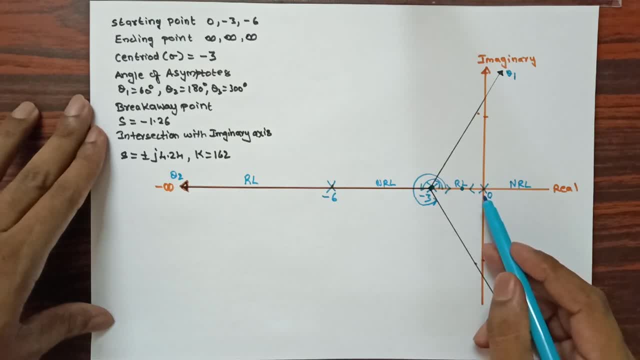 the value what you got, that you need to check whether you are getting within the root locus path or not. here the value i got: minus 1.26. you can observe here 0 to minus 3 in between that i am getting s is equal to minus 1.26. the second value i got, s is equal to minus 4.7. that you can see here. 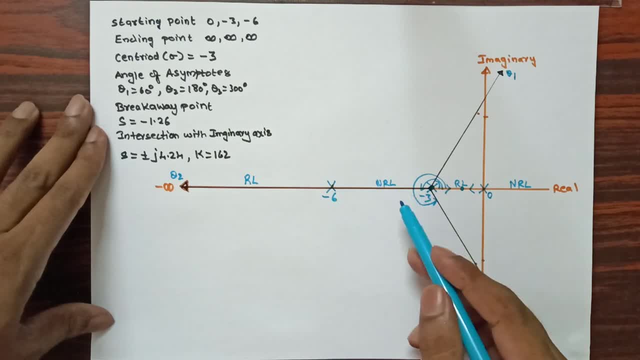 that i am getting in between no root locus path. that means by substituting in k equation we proved that it is invalid and here also in the graph also you can see that the value what i got, i am getting in no root locus path. so whatever the value of a breakaway point, you are getting in no root locus. 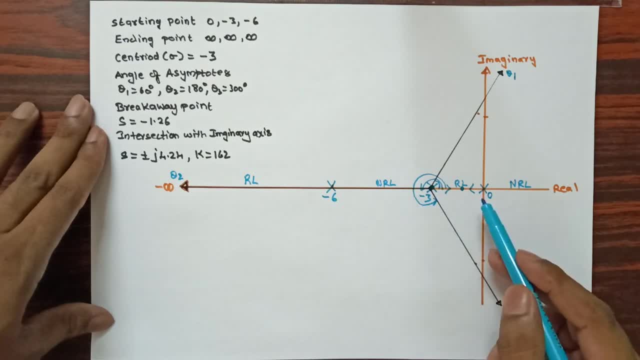 path. that is invalid breakaway point always will get in root locus path. therefore, this s is equal to minus 1.26 is a valid breakaway point. by observing in the graph also, we can check the validity of the breakaway point. now we know that this pole is moving in this direction and this 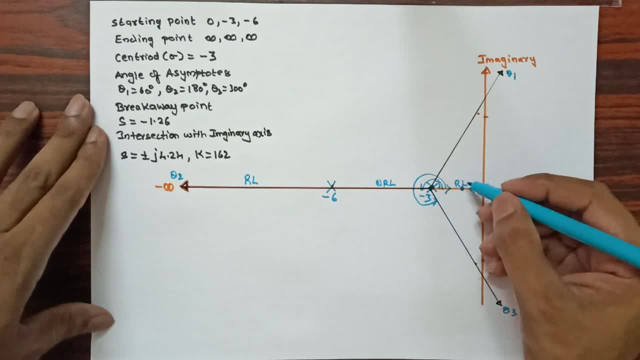 pole is moving in this direction. they are going to meet at this point and they are going to come out. one will come out in the other direction, in upward direction, and other will come out in the downward direction. now this suppose need to move towards to infinite path by following this angle, that is, 60 degree angle, and this pole. 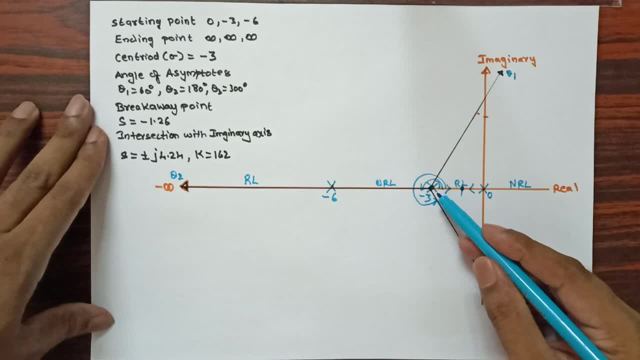 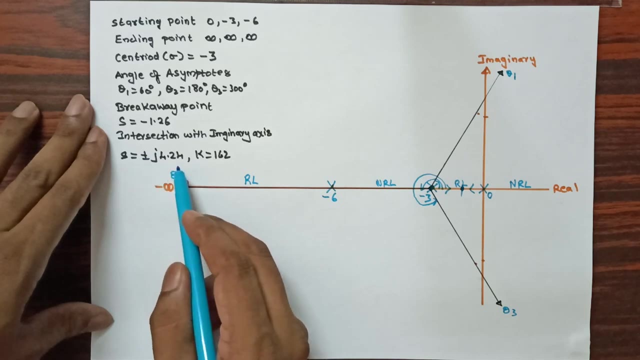 downwards pole is going to move towards to infinite path by following this angle, that is 300 degree. but when they are moving in this angle they are going to cross the imaginary axis. for that we calculated the intersection with imaginary axis values plus or minus: j, 4.24. 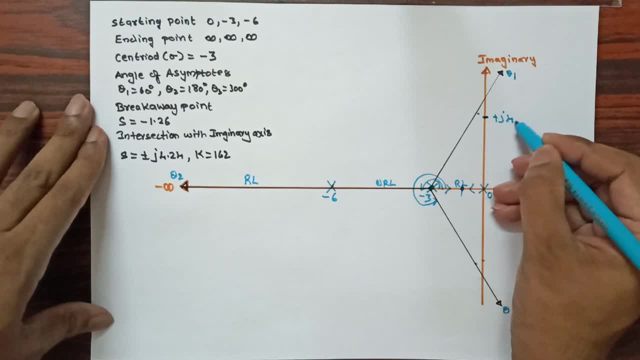 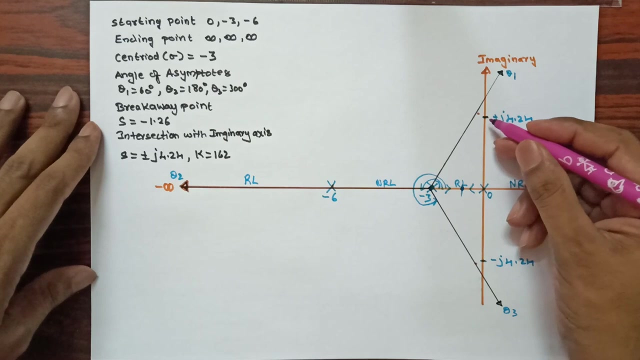 so here i am marking as a plus j 4.24, and at this point i am marking minus j 4.24. this intersection value i got for k is equivalent to 162. so from this point, the pole, by observing this angle and this intersection, it moves towards to infinite destination. the same way, this same way, this pole. 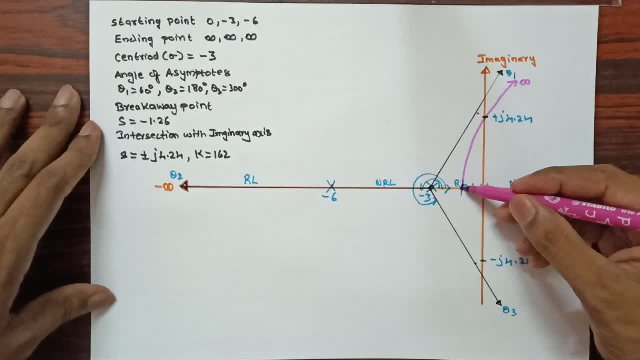 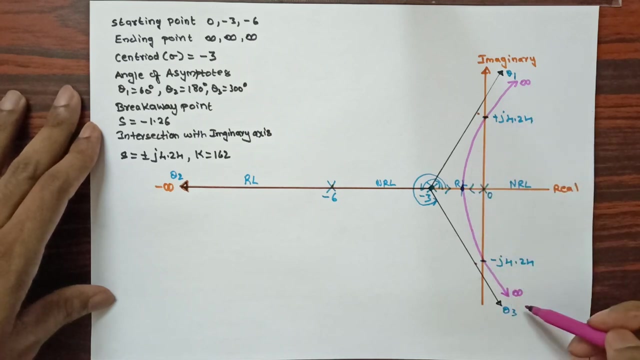 will observe this angle and this intersection point and will move towards to infinite path. so this is the locus we got. you can see here, this is the locus we got. it is symmetrical. you can see, in this, two poles have moved to infinite path. now the third pole, you can see this pole will be moving in root locus path in. 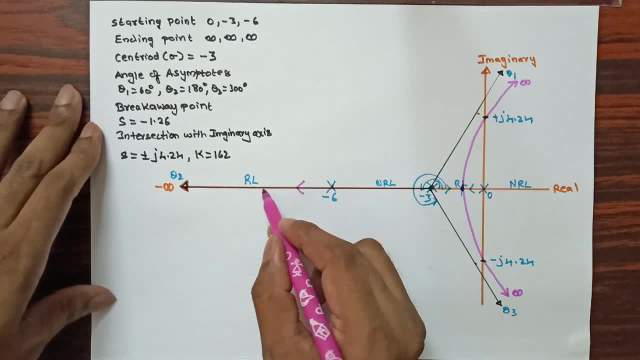 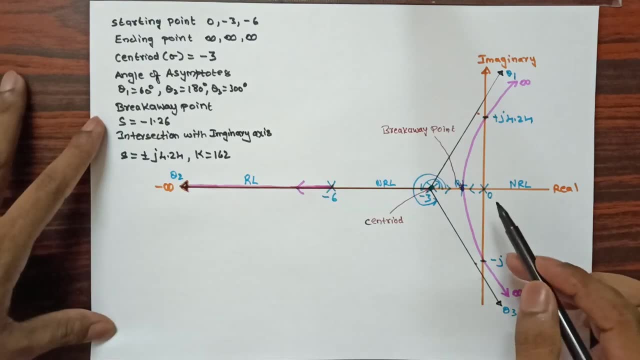 this direction and by following the 180 degree angle, it moved towards to infinite destination. this is the sketch of the root locus. in this you can see we have considered the poles 0 minus 3 minus 6, and then we have considered the center height point. at this point we have drawn the three. 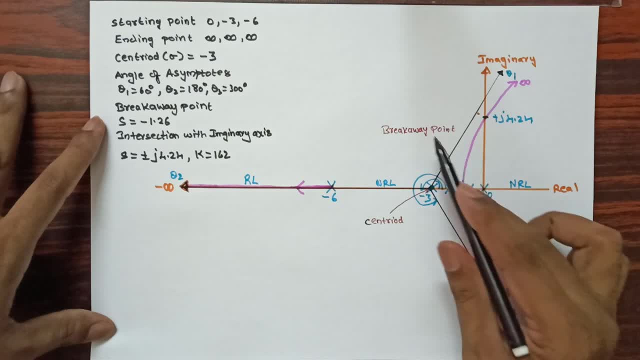 angle of asymptotes and then the breakaway point we have shown here, that is a minus one point two six. then we know that when we applied the input, the pole has been moved towards infinity and the pole have moved in this direction and this pole have moved in this direction and they have met at 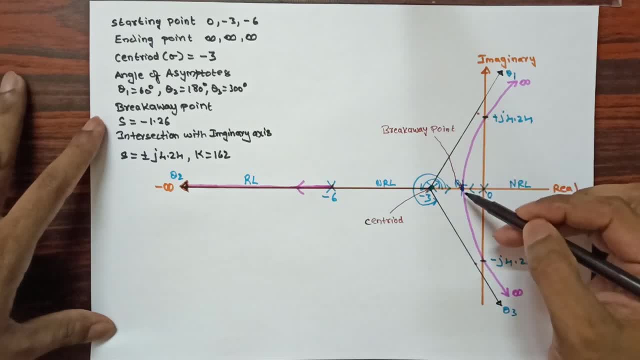 this point and observing to this angle and this intersection, the poles have moved towards to infinite path. and the other pole also. you can see that by observing to this angle and this intersection point, it have moved towards to infinite destination. and the third pole, in this case, you can see that it have moved towards to infinite at an angle, 180 degree, that is. it is. 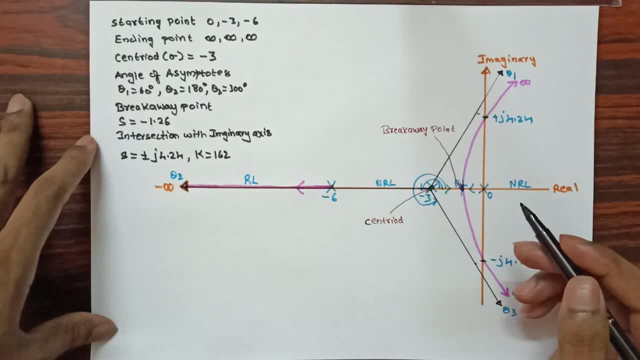 moving in the root locus path. now we are going to comment on stability. to comment on stability, we know that for an system to be stable, the root should be on the left hand side of the spline. if any root comes to the right hand side of the spline, it becomes unstable. now, in this you can